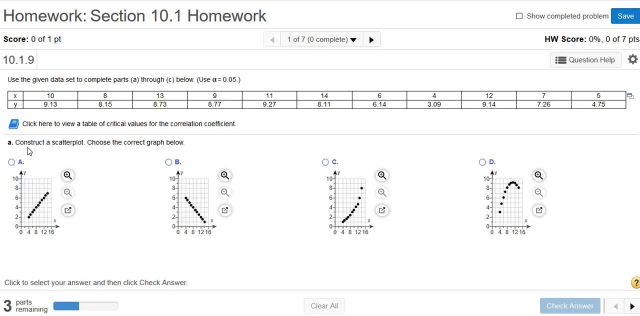 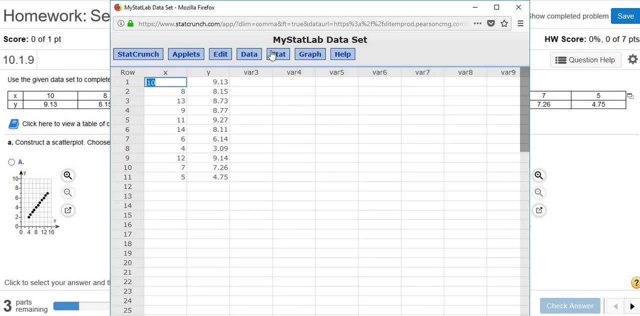 In this problem. we have a bunch of x and y ordered pairs, and the first part of this question wants us to construct a scatter plot. So what we'll do is we'll click on this little box here and select open in StatCrunch, And then we always go to Stat Regression, Simple. 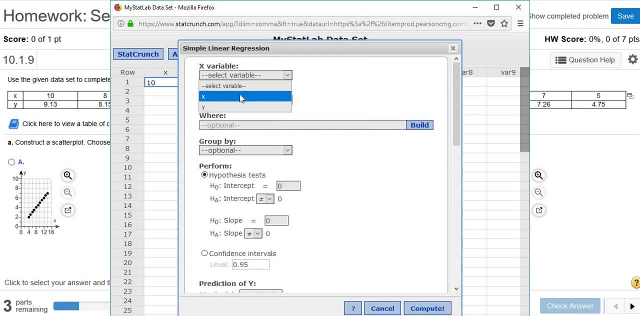 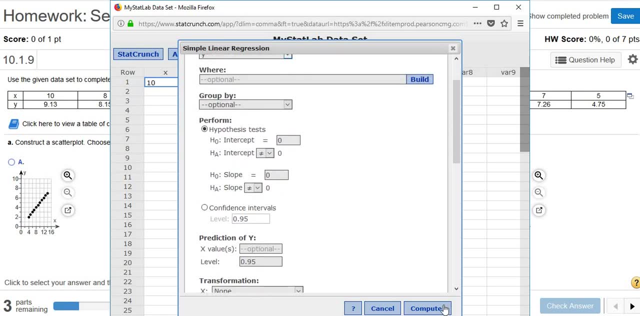 Plot. okay, left click and just always pick x and pick y, usually the first thing and the second thing And all of this stuff. we just leave it alone and click Compute, So you get all this information here. So where's the scatter plot? Ah well, if you click this, 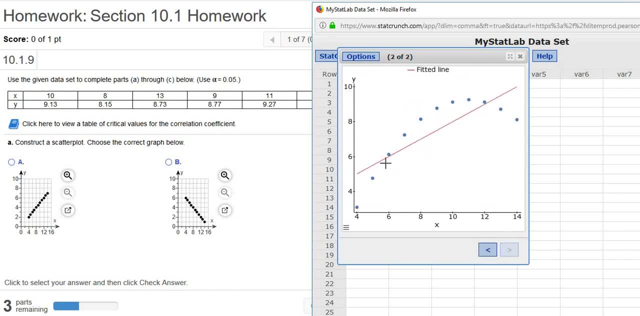 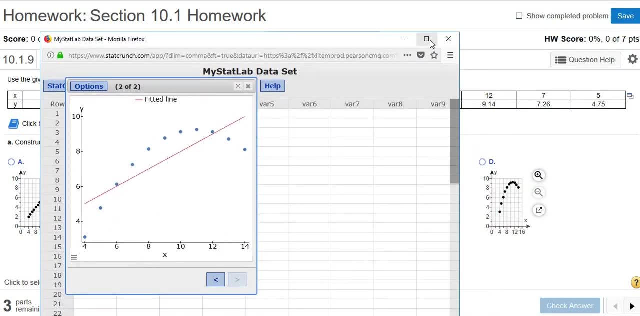 little arrow. here you get the beautiful scatter plot. So that's the scatter plot. Okay, so let's see if that's one of the choices. Yep, it sure is. Let me do that again, so you see it. So you click the little box, click Open in StatCrunch. 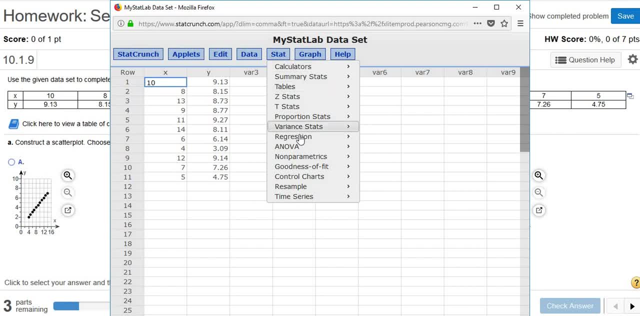 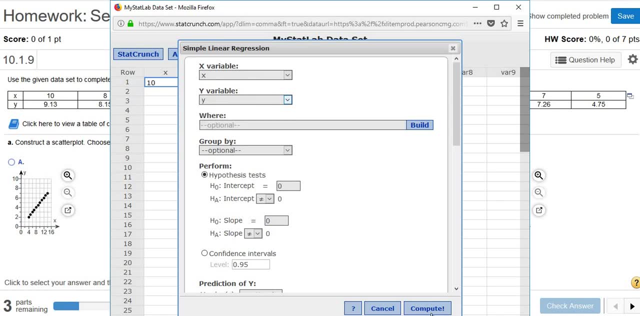 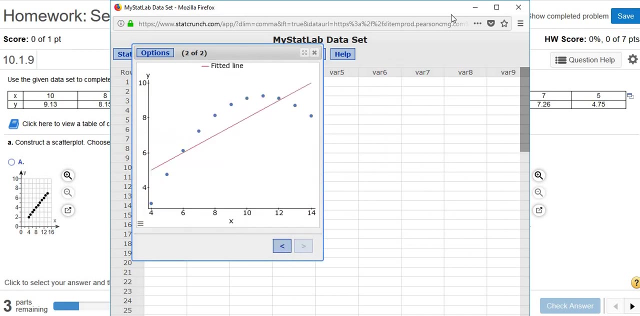 And you go to Stat Regression, Simple, Linear, Always just pick the first thing and pick the second thing. Ignore all of this stuff. just click Compute And you get all this information here which we'll use later. And just click this little arrow here on the bottom right. 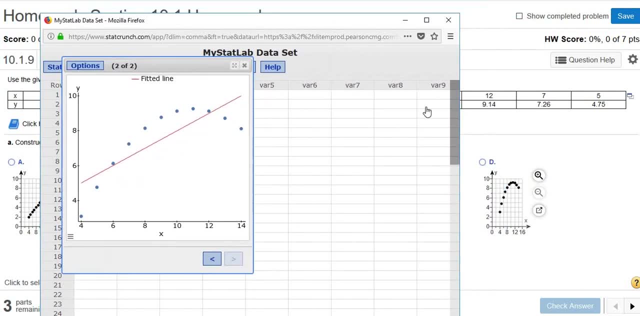 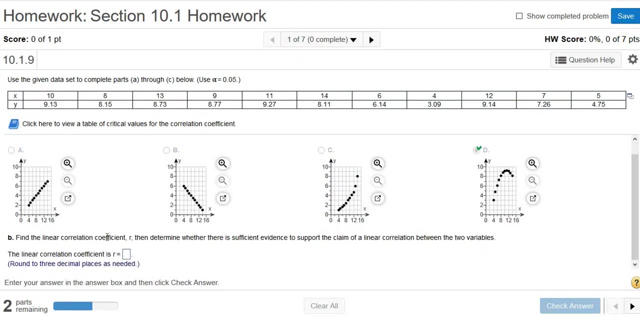 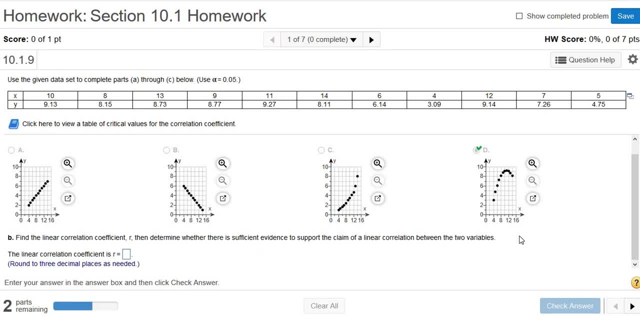 coefficient r, Then determine the linear correlation coefficient r, Then determine whether there is sufficient evidence to support the claim of a linear correlation between the two variables. So linear correlation between the two variables means that the data follows a straight line pattern. So we want to see if the data follows a straight line pattern. Obviously from the 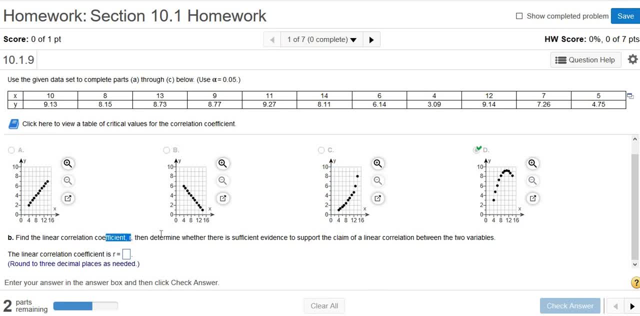 scatter plot. the data does not follow a straight line pattern, But this is a mathematical way to determine that. So visually it's not a straight line pattern Mathematically. what does the math tell us? Let's find out. So I'm going to click on this again and click. 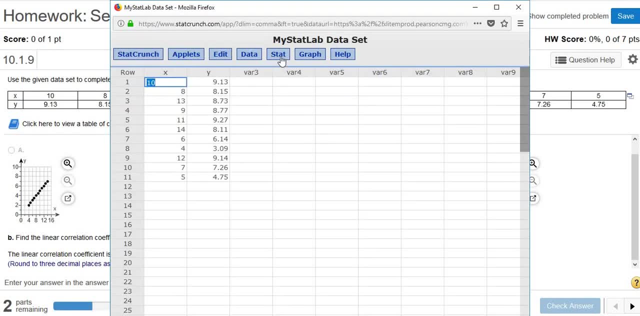 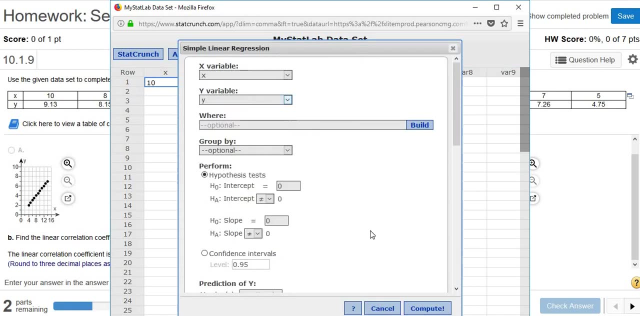 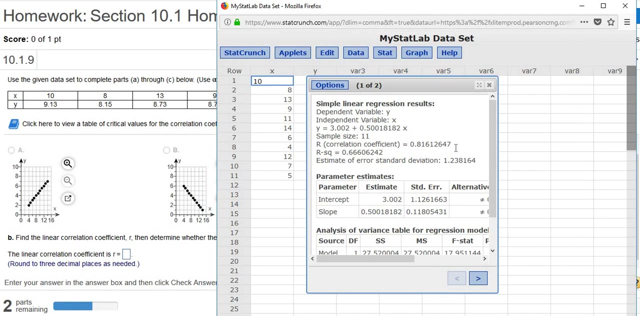 Open in StatCrunch regression, simple, linear, And again, just pick the first thing and pick the second thing, Click compute and we're looking for the linear correlation coefficient. We want three decimals. It's right there. There it is R Correlation coefficient. 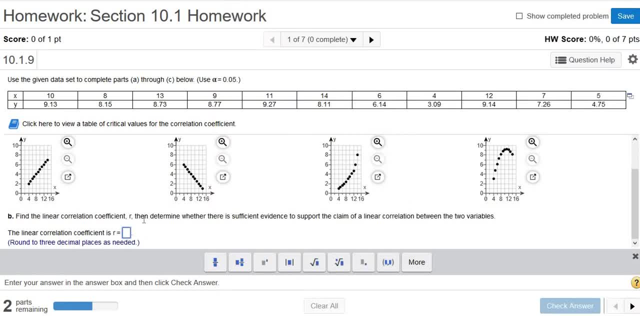 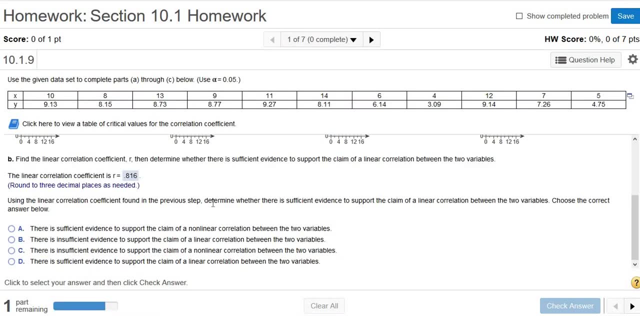 So .816.. I'm going to go ahead and type it in .816.. Good job. Use the linear correlation coefficient found in the previous step. Determine whether there is sufficient evidence to support the claim of a linear correlation between the two variables. Okay, so, in order to determine whether there is a 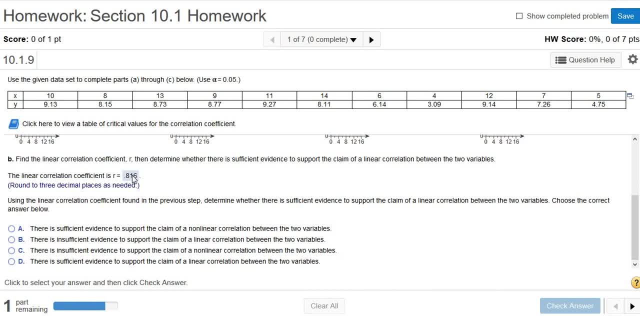 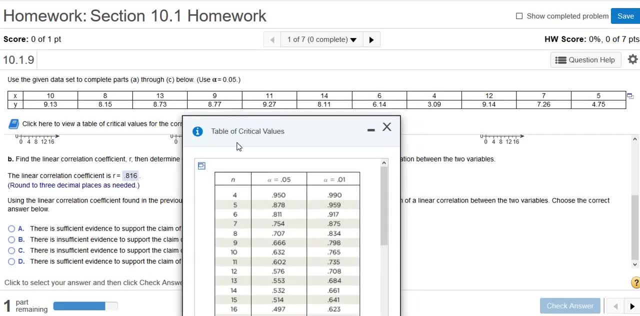 straight line pattern. mathematically, you have to look at something called the critical value. Okay, so once you find R, you click on this little box here and you get this table. How do you use this table? Well, you have an n and an alpha. 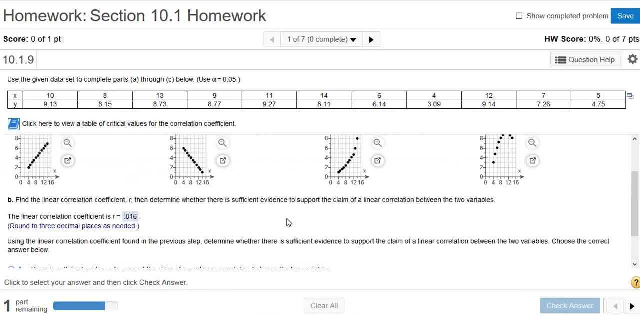 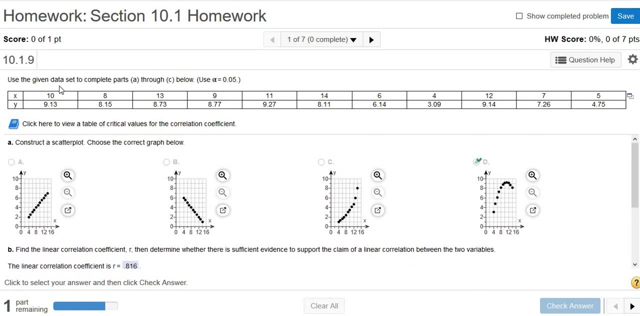 The alpha should be given somewhere in the problem. Let me look for it There it is up there. Alpha is .05.. Alright, so then n you have to count the pairs 1,, 2,, 3,, 4,. 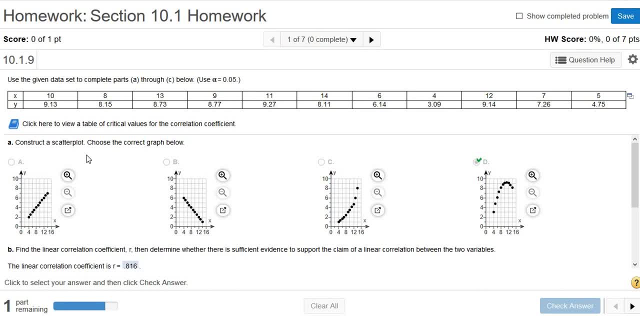 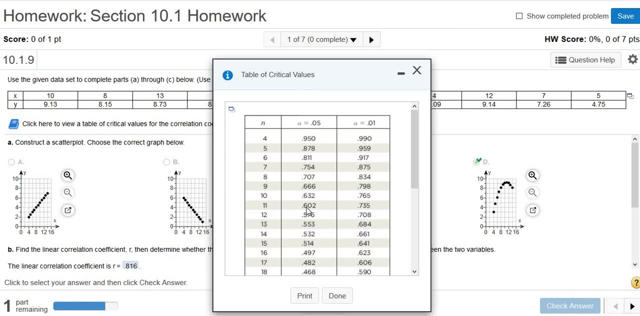 5,, 6,, 7,, 8,, 9,, 10,, 11.. So you click on this, So you go down to 11 and then your alpha So .602.. That's called the critical value. So if your R is bigger than this number, then the answer is yes. 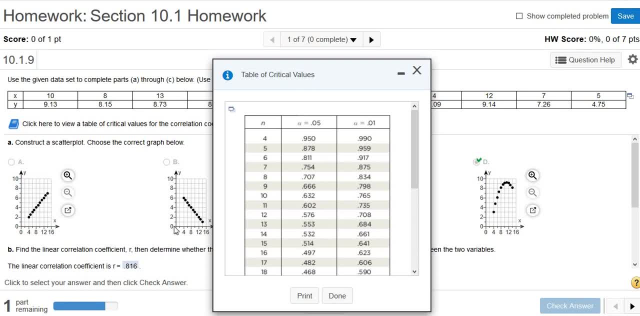 There is a straight line pattern. If it's not bigger, then the answer is no. So our R is .816.. So it's bigger than this number, So the answer is yes. Yes, there is a straight line pattern, So we're going to pick. 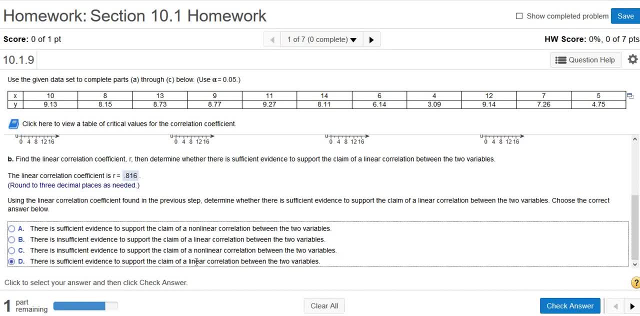 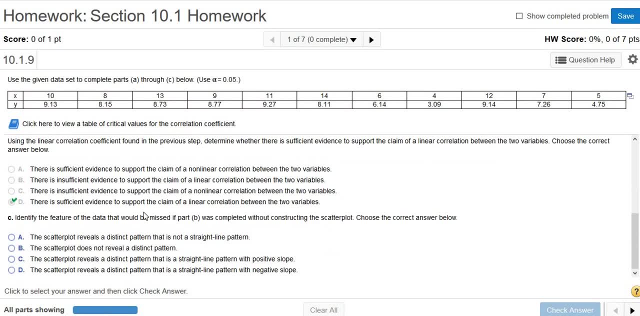 There is sufficient evidence to support the claim of a linear correlation. Okay, so yep, And if you have to guess, just guess. yes, It's usually yes. Identify the feature of the data that would be missed if part B was completed without constructing the scatter plot. 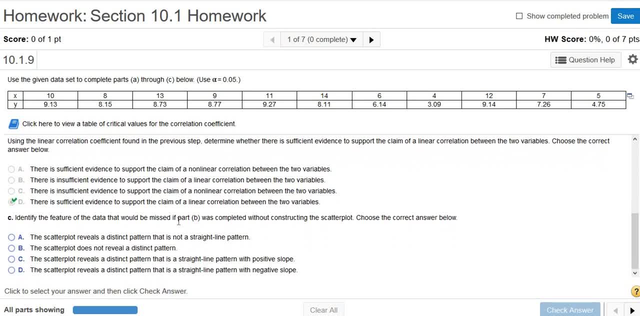 Yes, very good. So according to the math there's a straight line pattern, But this is not a straight line, right? It looks really weird. So I would say the scatter plot reveals a distinct pattern that is not a straight line pattern.